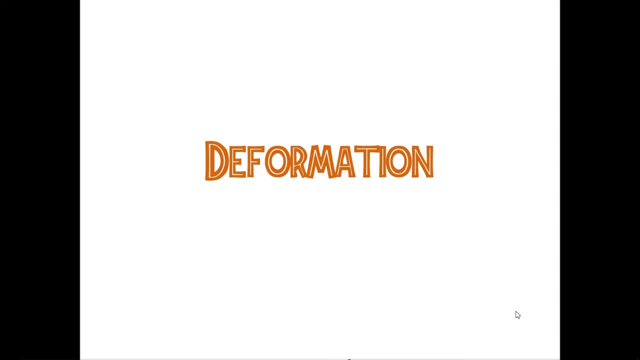 Welcome to the video lecture of structural geology, and I am going to start the first chapter of structural geology while discussing the deformation, Because most of the structures that we study in structural geology are as a result of deformation. Whatever they are, fold falls, joints. most of them are result of deformations, So we have to understand. 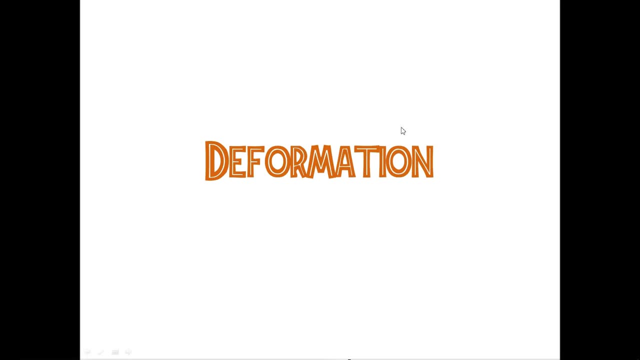 deformation first, before proceeding to the further chapters in structural geology. First of all, try to understand deformation with the help of this definition. Deformation is the transformation from an initial to a final geometry by means of rigid body translation, rigid body rotation, distortion, and we can, in simple language, call it distortion. 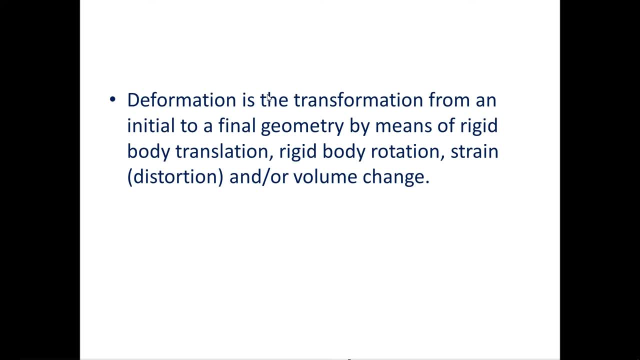 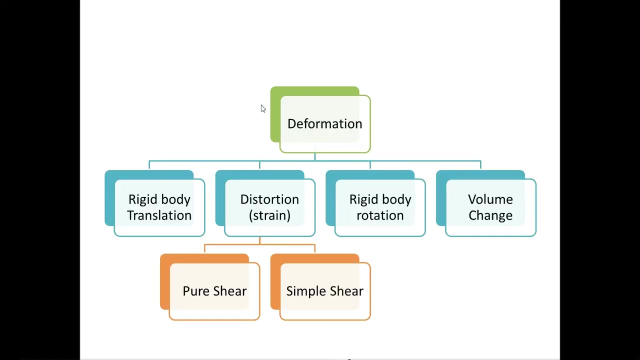 In a simplified version we can actually classify this kind of deformation and we can represent them As shown in this flow chart. So this deformation can be of basically four types. Rigid body translation: that means the body is not changing its shape, rather it is being translated from: 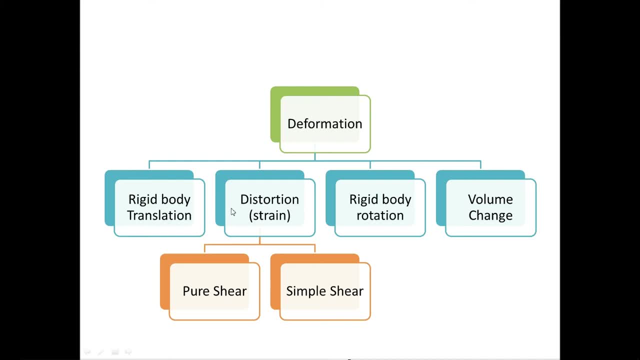 a position to another position, Then it is distortion strain. it can be further divided into pure shear and the simple shear. Then we have rigid body rotation. Here the body is rotated in its own axis and we might have volume change. So these 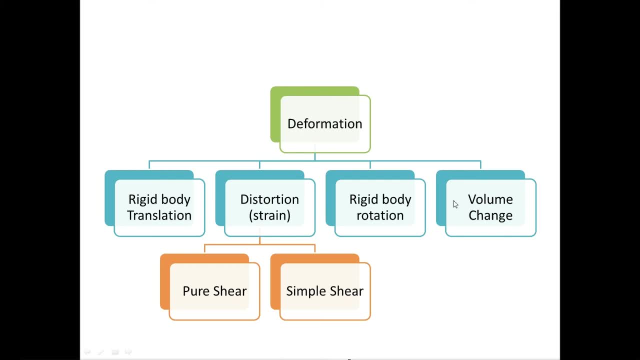 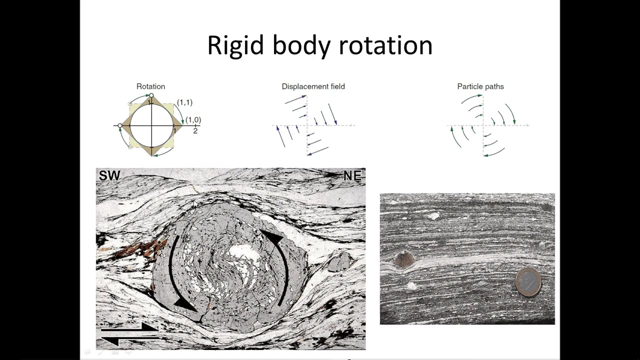 are representation of different kind of deformation that a body may go under deformation. We can call it body deformation if it's through any of them or a combination of them. So let's discuss about each of the kind of deformation one by one. First I am going to talk about rigid body rotation. As we can see here, the object which 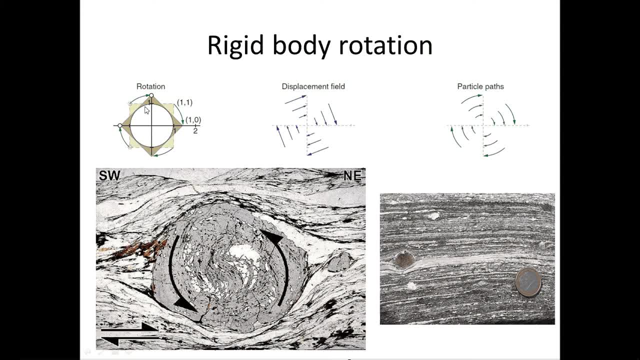 is in the light curve, this is square and it is rotated, So this point comes to this point, this point now becomes this point and, similarly, all the point. it is simply being rotated. No change in the shape, no change in the volume has taken place. 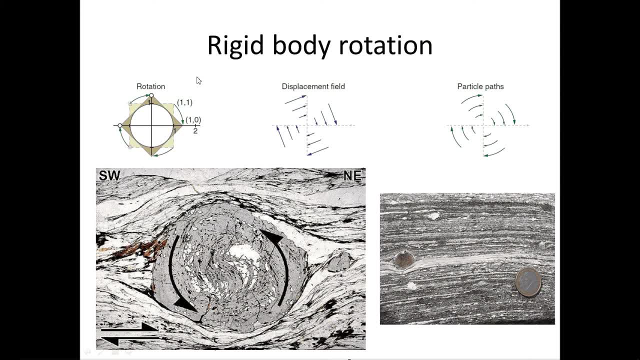 so this is the rigid body transfer, rigid body rotation. so when a body do not show any volume change, any shape change and just rotate in its axis, we called such deformation as rigid body rotation. and these are this. these vectors are showing displacement field and these these vectors are showing the path of these. 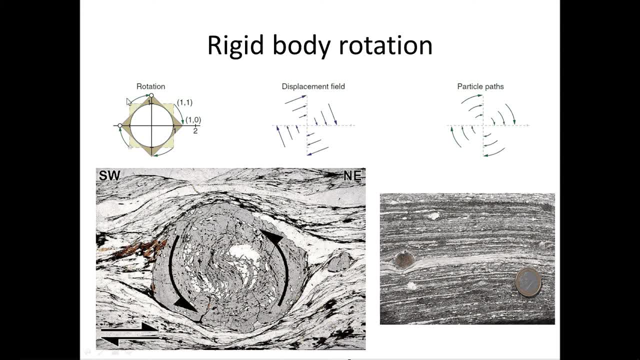 particles. okay, and how this can be made is represented in this diagram, so this point is migrated to this point. okay, while rotating, and this the rotation, rotating axis must be at this center position and it will be perpendicular to this screen. okay, and the example of such a rigid body: rotation. although here I 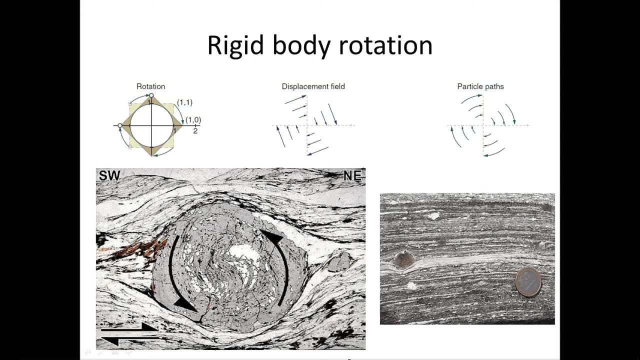 have shown example of a garnet which has been rotating, although it is not a rigid body rotation, as we can see a bit of deformation in this shape also. so we can't say it is a proper rigid body rotation but it is an example of rotation. so we know that rotation is is a deformation which is possible in rock. 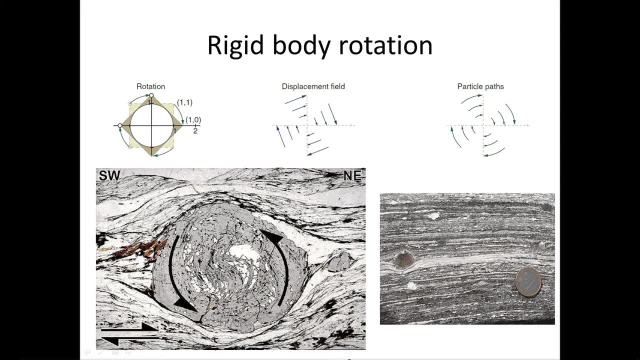 so you don't have to be in a fluid medium to a particle. okay, so rotation can also be achieved in a solid state rock. we do study the flow of the particle of, or the flow of the grain in the rigid bar, in the rigid body or in the solid body, and it is come into the topic rheology and 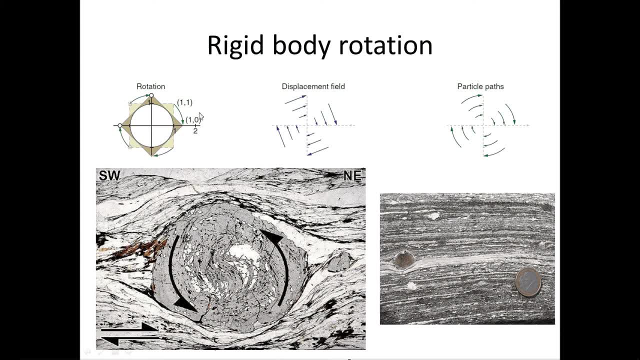 we will discuss it later, in the later chapters. okay, but for now we can take the example of corner. this is the rock, some metamorphic rock. it appears to be nice, okay, and in this nice, we have this garnet. okay, and when we see this garnet, 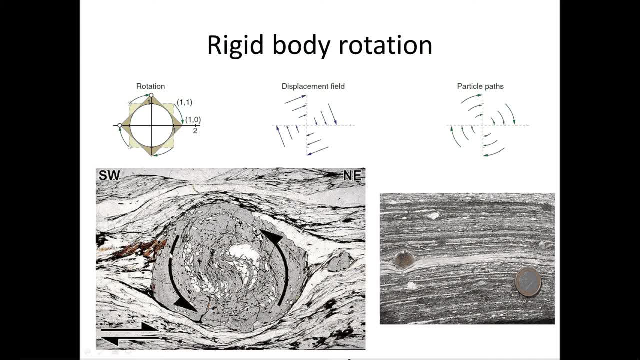 in plane polarized light, in petrography. when we do the petrography and look at this garnet in plane polarized light, we can see the garnet, this fleshy color garnet, and we have inclusion of quartz and this is also a very nice shear sense indicator. so this is the dextral kind. 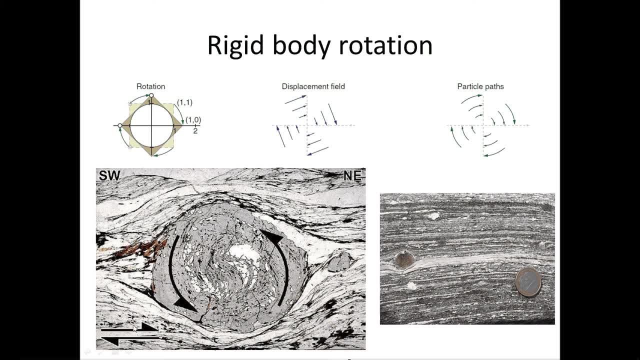 okay, so now this is the. it is the sign convention. it is sinister. the grain is rotating sinisterly while the deformation is going dexterity. okay, so the although all over the flow over the rock is dextral, but the grain is rotating in its opposite direction, which is sinister. 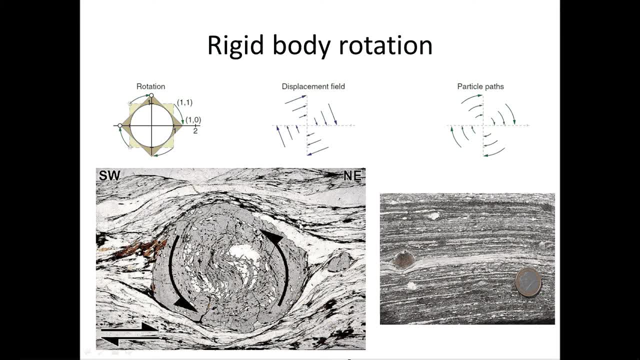 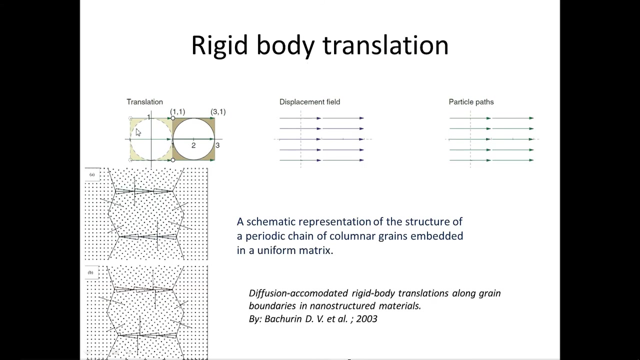 okay, so this is the rigid body example of grain rotation, although it is not a rigid body rotation, so we can. it is also possible that if a very competent grain is showing rigid body rotation during deformation of rock, so this is a possible case- then we come to rigid body translation. if you put an object which 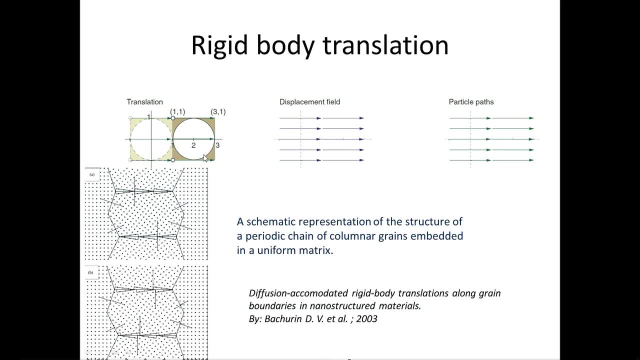 initially at some point and place it to another place. okay, another position. this kind of deformation is known as translation. in the translation kind of deformation there is no change in the volume, there is no change in the shape and there is no rotation. it is simply translation of. 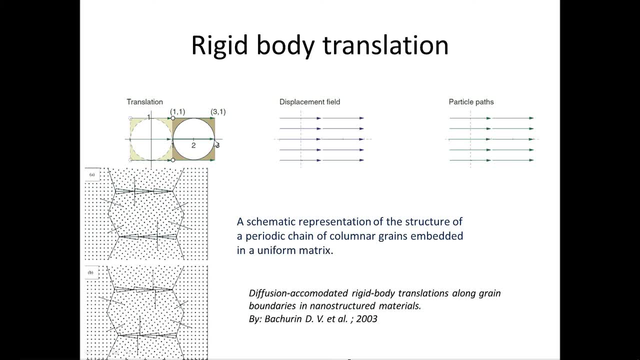 a particle from one place to another place and we can show the displacement field like this and the particle, the path of the particle, is straight. these are not making any curve circular path, because it is because there is no rotation involved here. so it is a simple translation and these translation is not 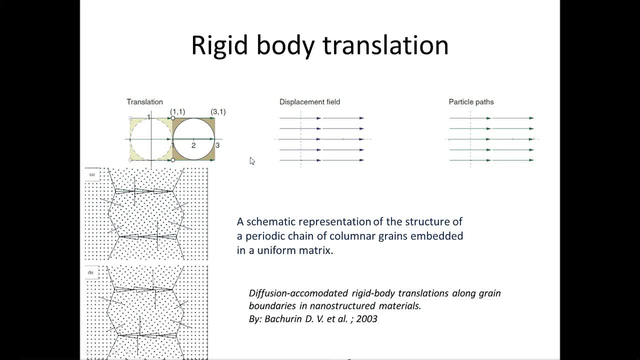 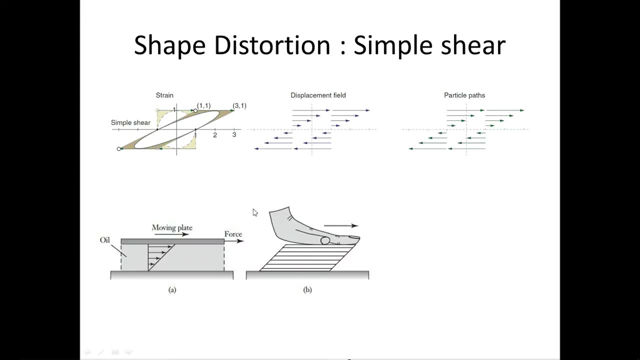 basically seen by a very large size grain that we can easily observe. but yes, this is this rigid body. translation is also possible in the rock and, although not very common, then we come to shape, distortion, simply distortion, or shear, we can say it is as we can see. 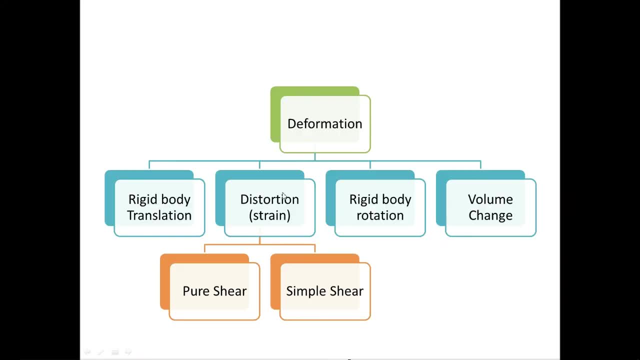 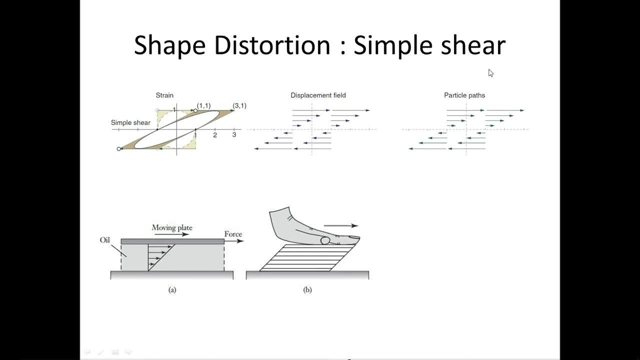 from the flow chart diagram that distortion or the shape distortion or strain accumulation, this kind of deformation, okay, can be sub classified into pure shear and the simple shear. so while discussing the distortion- shape distortion- at first, I am going to talk about the simple shear. look at this: figure a and b. 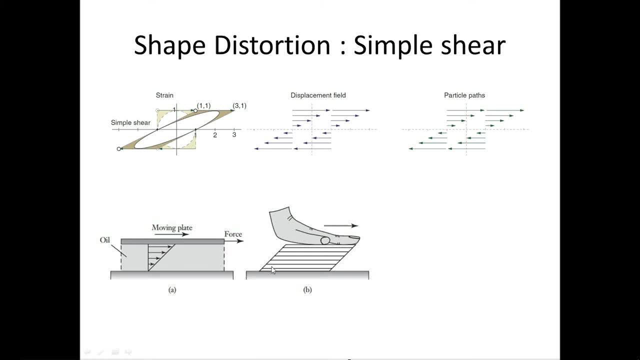 suppose you have a deck of cards and you put your hand like this and slide it, so the deck of cards will result to be the deformed in this manner. okay. Similarly, there is an another planning question about the distortion of this work to Oh, while discussing the shape distortion, and I am going to talk about the simple shear, Look at the figure. to whites above, say, if you have a deck of card like体 and you put your hand and slide it, so the economy has a hole middle background, and if you have no of card, similarlyts also it служ on earth. 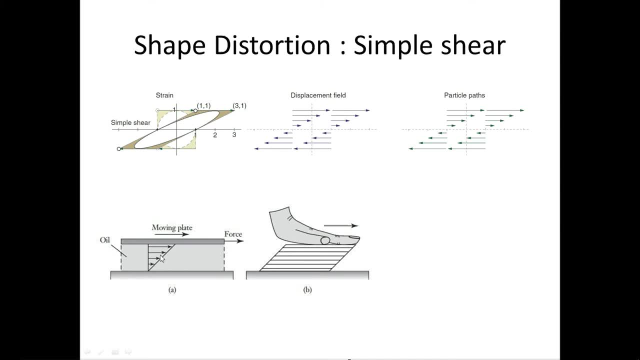 this is a plate which is lying over oil, okay, and you are making a force so that displacement would be like this. this kind of deformation result in the distortion of the shape of the body. so at first this deck might be rectangular in. this deck of card must be rectangular in shape. but when you slide it and 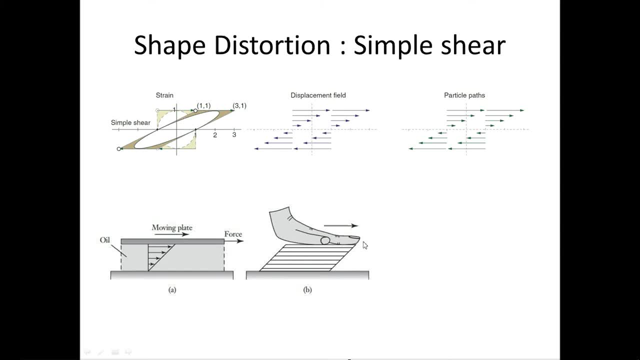 deform it, it will become rhombus in shape. parallelogram: rhombus in shape. okay, now, this is a simple representation. this was this square. okay, and in this square you can see an inscribed circle. okay, in the light shaded region you can see a square and within this square you have a circle. 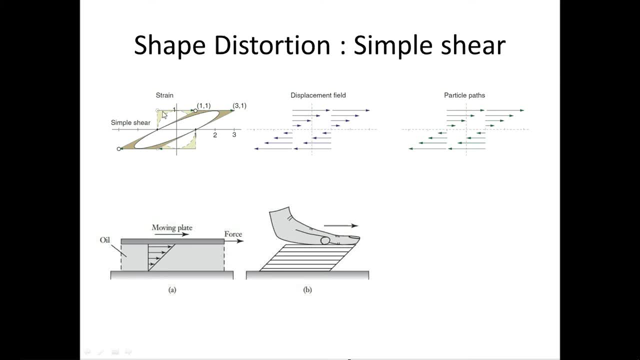 and when you slide this, you do you make a for when you apply a force like this, parallel to these, this x-axis here, okay, like this. so the body will deform in this manner. okay, elongated to this, these two diagonal point and shortening will be in these two points. okay, these two point will test to shorter. okay, that is. 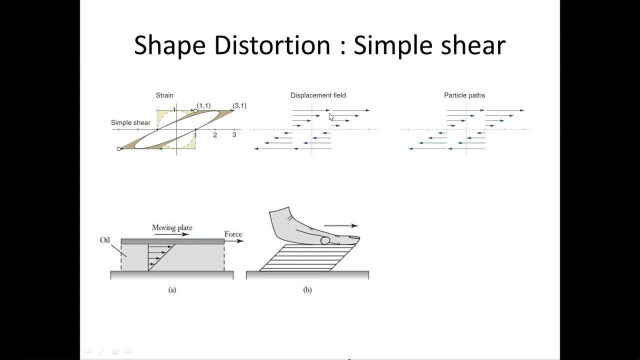 field would be like this, somewhat like this, and you can clearly see. if you make this, this, you can see the field where it is deformed. so this is the maximum strain accumulation axis where the maximum extension is taking place along this, from this point to this point, if you connect this point, a diagonal, this: 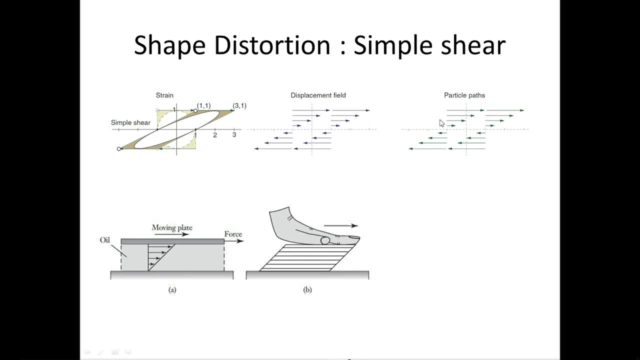 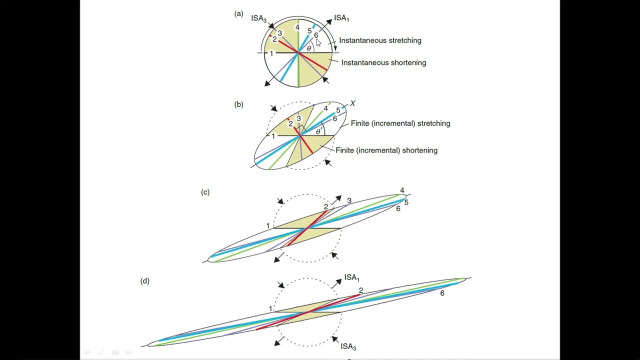 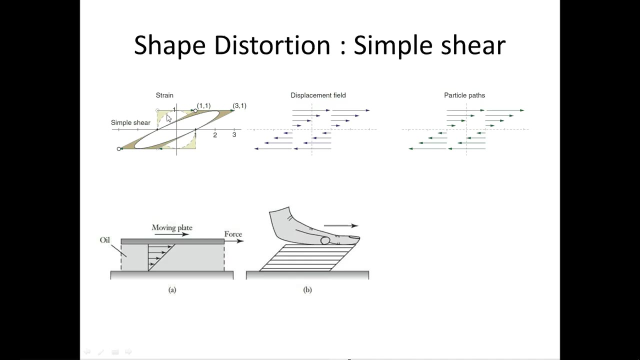 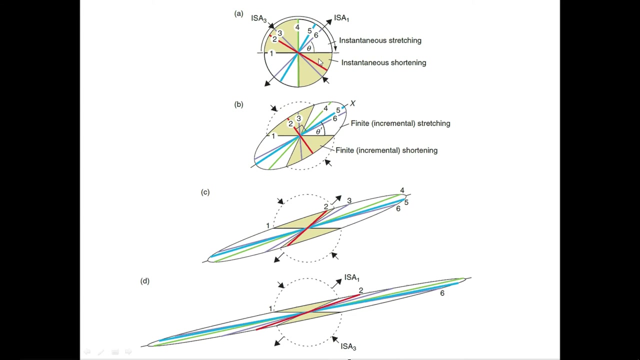 diagonal will be the maximum extension showing the. this is the path of the particle and here we can see the regime. okay, so in this region, this we can divide the whole circle. the circle was present in an undeformed body. okay, so this is the circle representing the undeformed body. now, as the strain is, 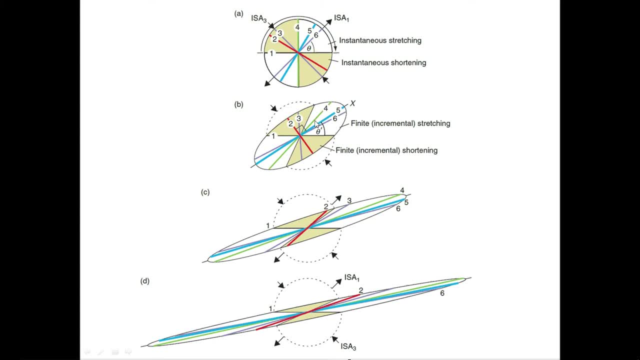 accumulating, the body is being deformed, the circle is picking a become is becoming影片. elliptical that means elliptical shape. okay, so it is becoming more elliptical, more and more elliptical and becoming elliptical shape. okay, so this white regime is showing the extension of this stretching regime, while this creamy 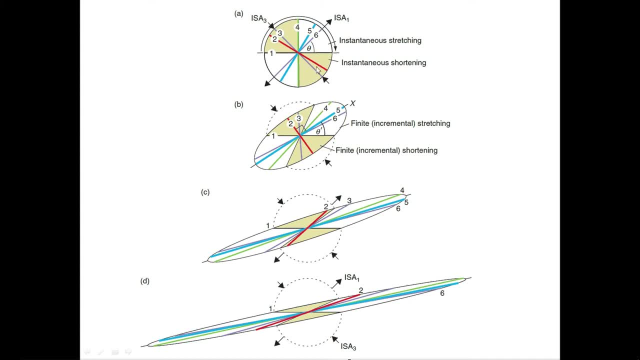 layer is showing the shortening, the shortening regime, where the lines, material lines are going to be shortened. okay. so if you put a material line in this creamy layer region and after deformation you can find that that material line developed fold. okay, because the shortening is taking place. 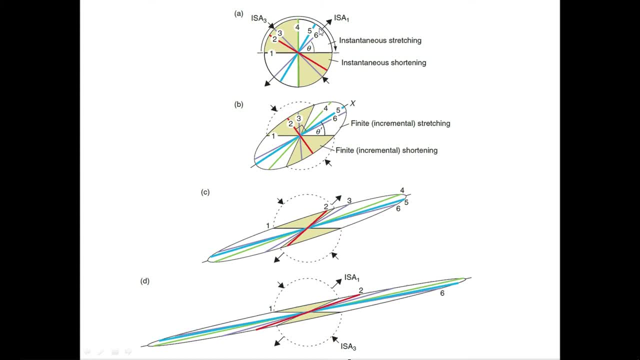 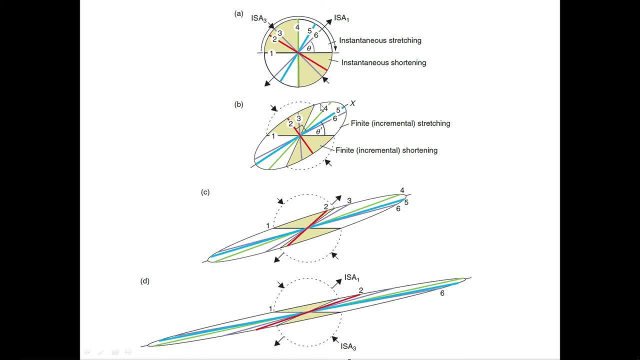 So it is the axis where maximum shortening is taking place. As you can see as gradually this circle is becoming deformed because of the applying stress over it, It is gaining strain. Moreover, it is rotating. So it is a non-coaxial deformation because the axis are rotating. As you can see here, the position of these axis are rotating. These are trying to align along this line 1.. So you can see this line 1.. This is the line 1 and force is being applied in this. parallel to this, 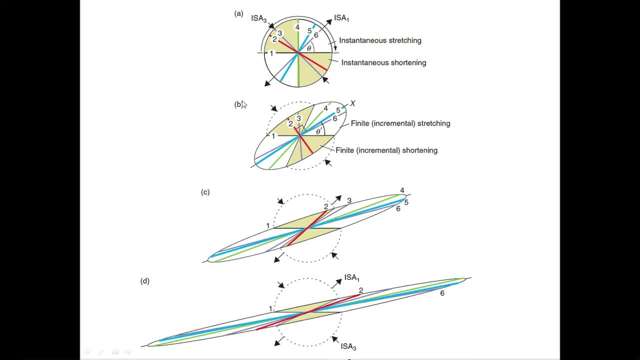 It might be, it is, it must be Dextral. Okay, It is, try to orient dextrally. We are making, shearing it. and that force line is parallel to this axis 1.. So all the material line are trying to orient themselves along this 1, along the try to orient themselves parallel to this line 1.. Okay, 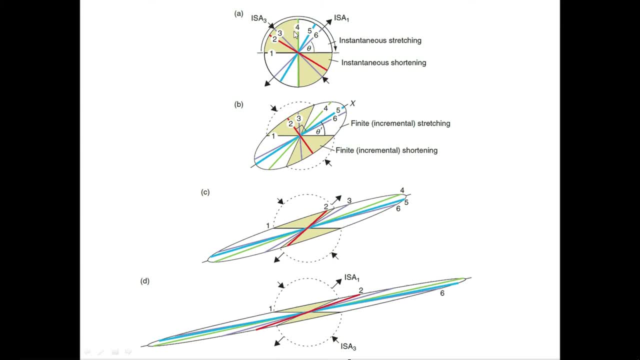 So, initially, this line, this 4, just look at this line 4.. It is, at this position, perpendicular to the line 1.. But as the strain is being accumulating because of the increasing stress in the body, It is this line 4 is try to orient itself parallel to the line 1.. 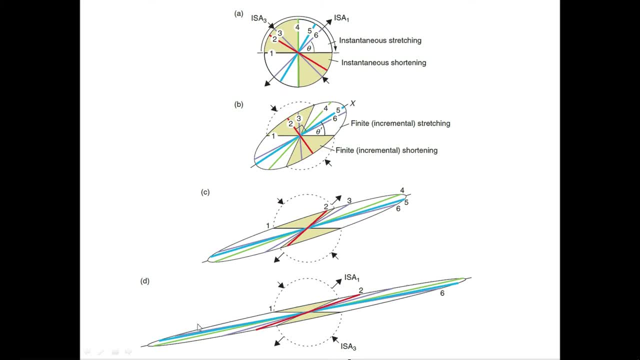 So this is highly deformed, highly deformed ellipse here and you can see here the axis 4, the green color is being rotated. So this is an example of non-coaxial deformation And this non What is non-coaxial deformation? 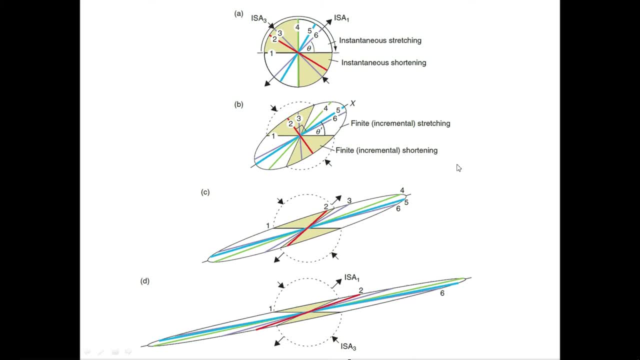 And this non. What is non-coaxial deformation And this non? What is non-coaxial deformation? And this non-coaxial deformation, Non-coaxial deformation is a kind of deformation in which the axis or the lines that are storing the strain, in itself they are actually rotating. 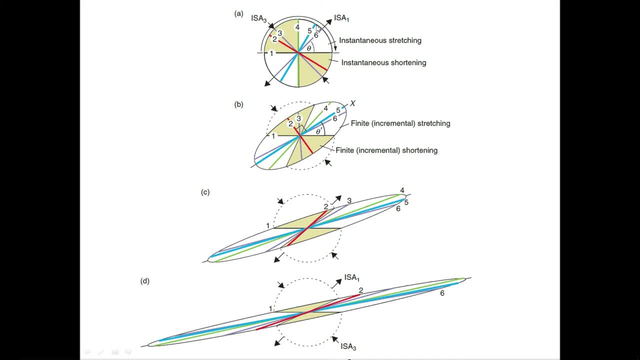 So here the axis, the strain gaining axis, are rotating. that means it is a non-coaxial deformation. Okay, So 1 is the only line where there is no deformation. There is no deformation. Okay, As you can see here that the length of the 1 is not changing. 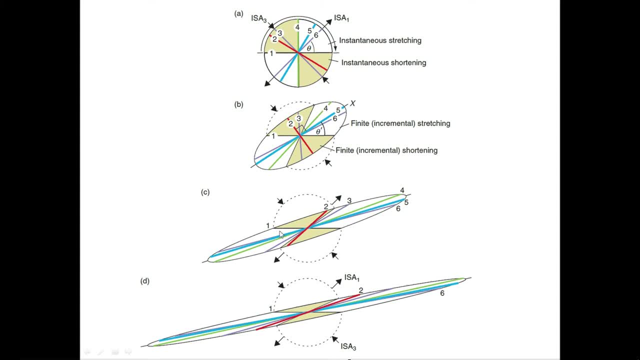 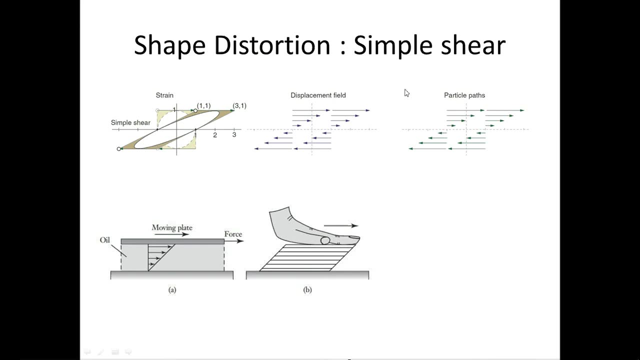 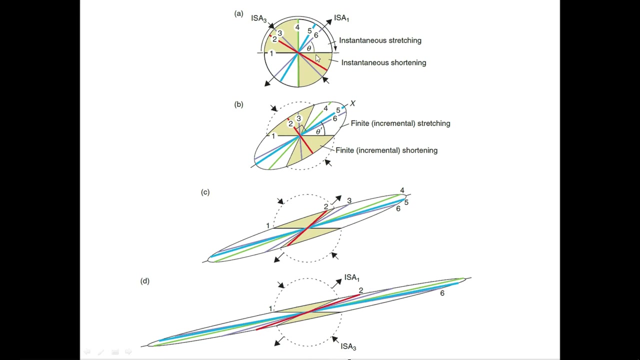 Length of the line 1 is not changing. moreover, the it, the 1, the line 1 is also not rotating, So it has the only line in the simple shear, this one line, that is the line which is parallel to the vector of force being applied to this body. 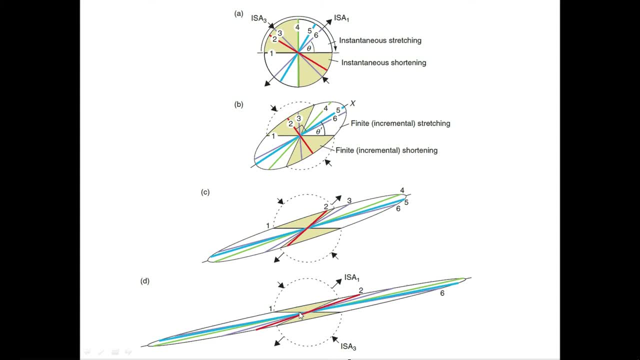 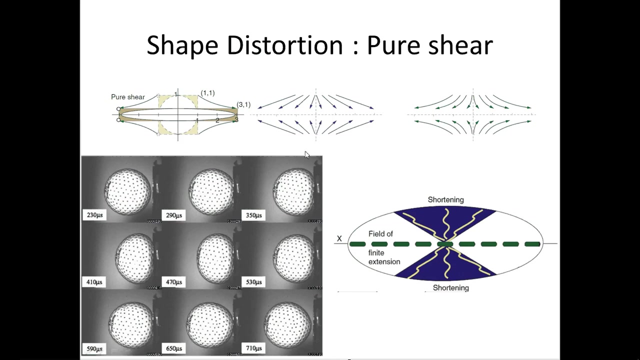 So this line is not deforming, It is not showing any deformation, It is not showing any strain. moreover, all other lines are try to orient themselves parallel to this line 1.. Okay, After simple shear, the another kind of shape distortion is pure shear. 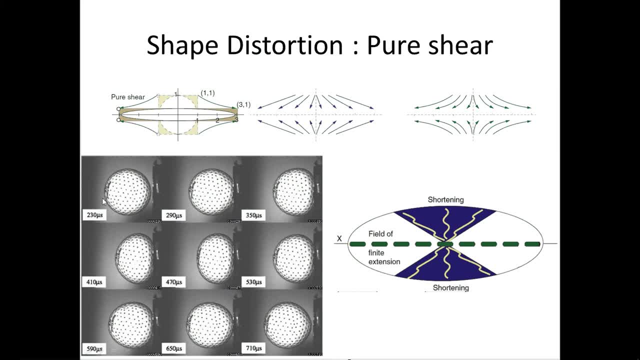 Look at this golf ball. In this, in this condition, at this stage, the this golf ball is perfectly spherical in shape. After this, this is 230 microsecond. after 290 microsecond, it just hit the surface. Okay, As soon as this ball hit the surface, you can see it is no more be a maintain its spherical shape. 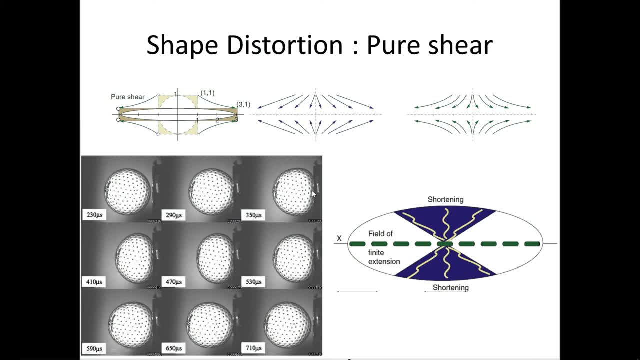 Okay, It is, it is deforming itself. Okay, And it's 410, 410 microsecond. It is becoming more and more elliptical. 470 microsecond, It is further more elliptical. Okay, And again it is. try to rebound. 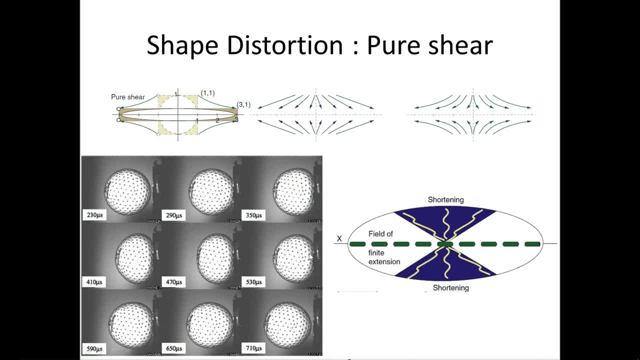 Okay, And during rebound it is again: try to restore its original shape. Okay, Which is spherical. So it this shape, this condition is: try is matching with this 410 microsecond. Okay, This 530 microsecond is somewhat like 410 microsecond. 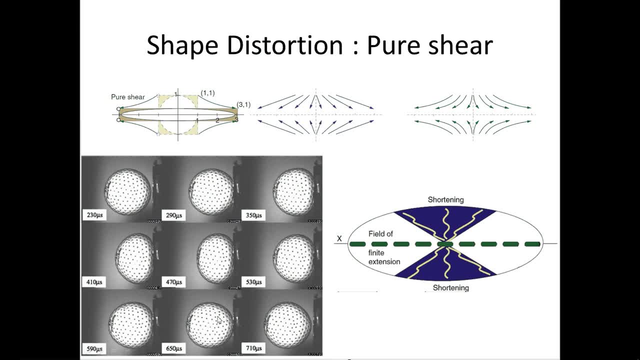 Okay, So the maximum deformation is at this state and slowly it is recovering and again it becomes spherical. Okay, So it is a elastic body, This golf ball behaving elastically, deformed and then again regain its shape. Okay, But when it was deformed, you can see it has it from spherical to it becomes an ellipsoid. 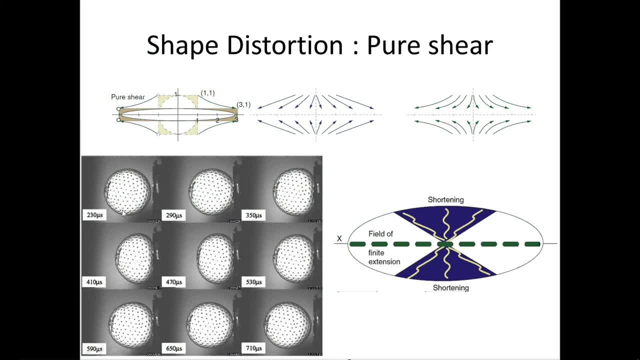 Okay, So, but in two dimension you can, it is looking like a circle which has become ellipse. Okay, Similarly, When this, this is the So, this is your initially, your body is like this: this square, and this square is inscribed in this square. you have inscribed circle and you apply a force perpendicular to it. 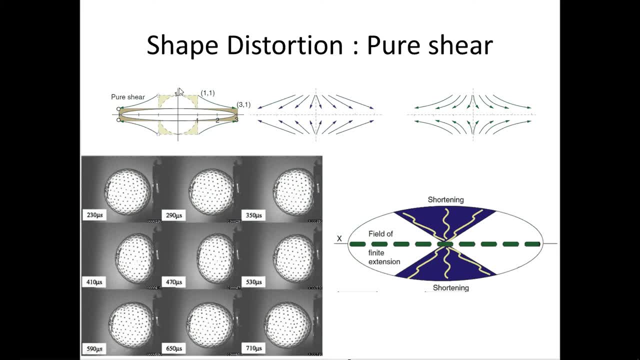 Okay, That is parallel to this line one. Okay, This is your maximum principal stress axis. You are making applying a force parallel to axis one, And you are, then there will be a deformation. Okay, So this body will no longer be a square, rather it will become a rectangle, and this inscribed: 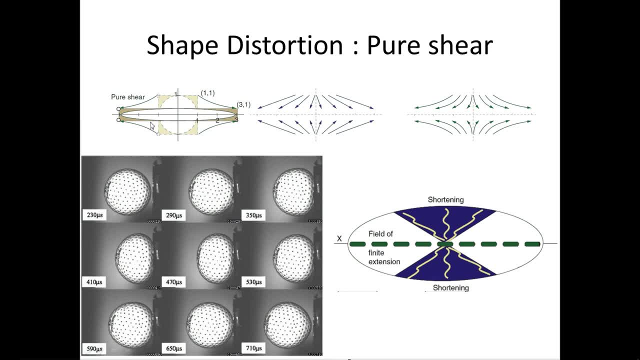 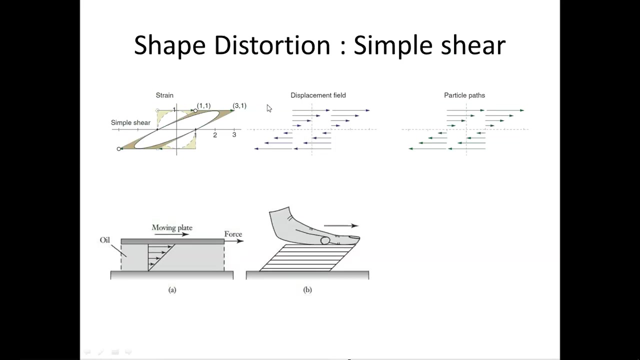 circle will become ellipse in shape, Okay, And the and this, this is extending in the direction of the minimum. the maximum extension, maximum strain will be in the direction of minimum stress. Okay, And if you look at the flow direction, Okay. Displacement field: 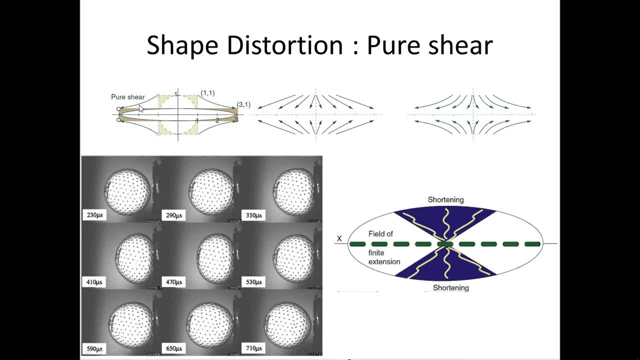 These lines would be like this and if you look at the path of the points, they will make a curve path like this: Okay, Although you can see, see here that if you suppose, if you have the this line one, Okay, So if you have a material line parallel to the line one after deformation, they have to. 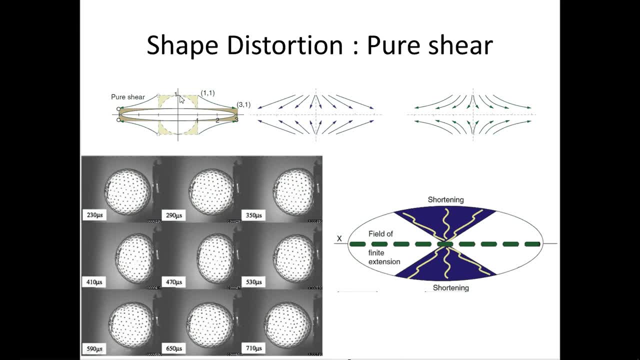 be shortened, Okay. So if I am starting, if initially I have a line which have is starting from this point to this point, after deformation, this had to be limited from this point to this point. Okay, So the shortening will be taking place in this regime, while the extension in this regime. 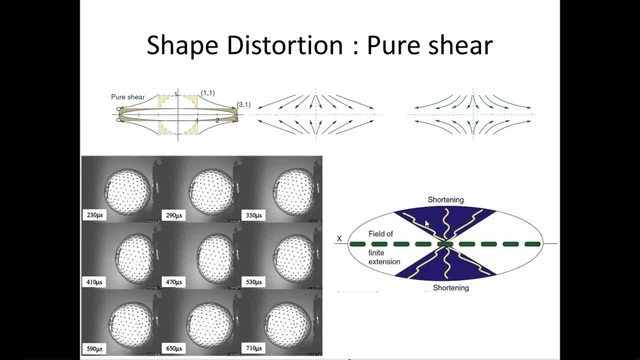 and this can be shown with the help of this diagram here. Okay, So this blue color is indicating the regime of Shortening, while the white field is showing the regime of extension. Okay, And the maximum shortening will be will be parallel to this excess one. 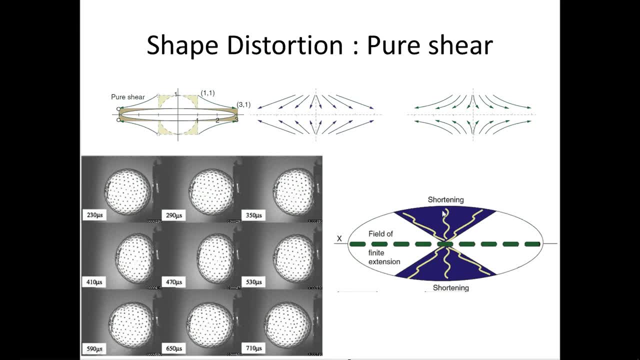 Okay, So this, this is the excess of maximum shortening. So we, here, we are getting fold and as we have material line which is as the material going far away or ending far away from this, This excess, there will be less and less and less and lesser accumulation of the strain. 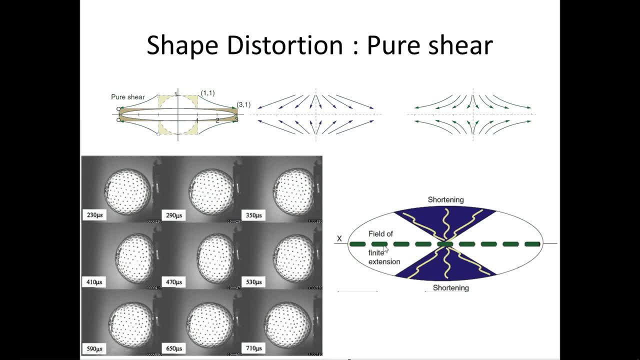 in them and they will develop less intense fold. Okay, Similarly, this X axis- Okay, You can see here X axis is the maximum extension- is taking place. So maximum shortening in this direction, Okay, Parallel to the one maximum shortening. 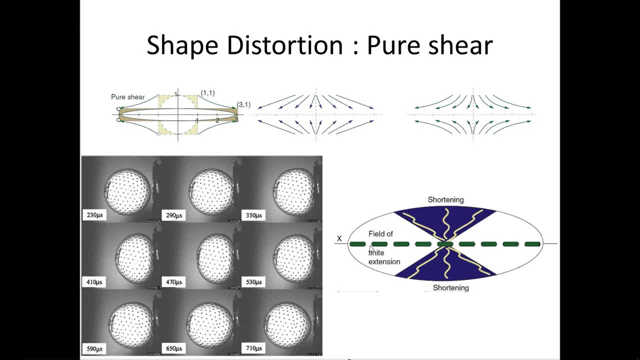 While the maximum extension It's just perpendicular to it And this is forming the body knowledge structure, as you can see here. that Okay, So so, as it is moving from the maximum extension towards the maximum shortening, So the intensity of the extension will gradually decrease. and these are the point. 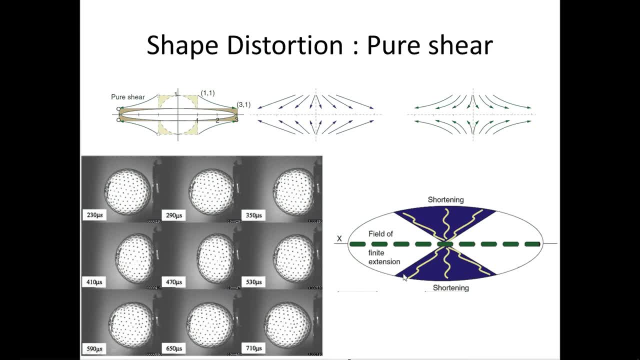 These are the point, these diagonal points We are did. these two regimes are meeting at this point, These material line. They will neither show any shortening nor show any extension, because it is the boundary of the regime of the shortening and the extension. 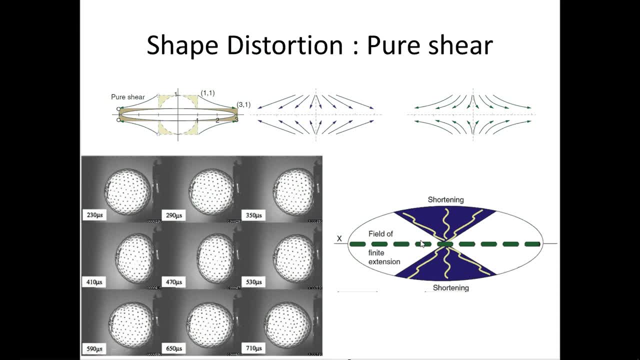 So these material line will neither show any shortening nor show any extension, So these can be called as excess of no finite change, Okay. Moreover, If you have an, if I have an material line which is parallel to this Axis one, Okay. 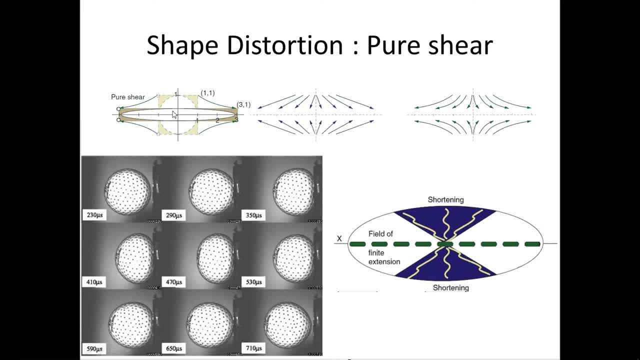 So it will not rotate in this pure shear. Okay, They will remain in their original position. position: They will not rotate. Similarly, if you have this axis, this x-axis, Before deformation and after deformation, they will not rotate, Okay, So this kind of deformation is called as coaxial deformation. 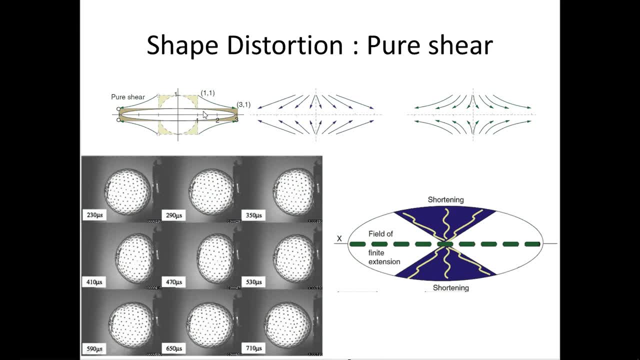 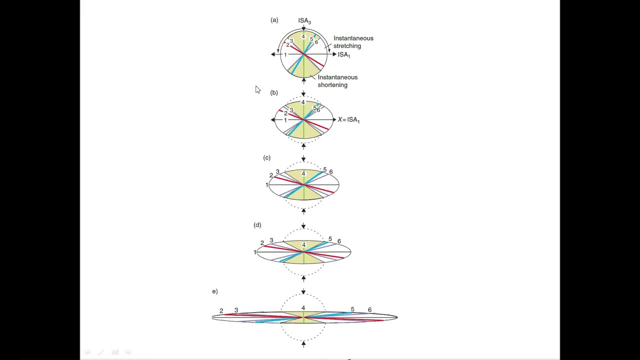 Okay, So in the coaxial deformation- Coaxial deformation- There will be no, There will be no orientation or rotation of this axis, And this is the diagram where we can see the strain accumulation. So is a three. Okay, I said three. 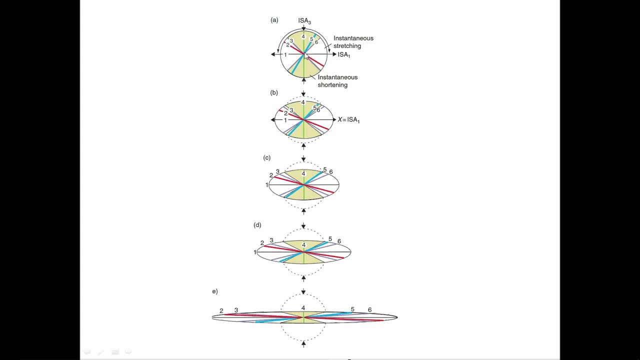 It is indicated, It is parallel to the axis for green one. Okay, So I said three means: the instantaneous. instantaneous shortening axis, Okay, And it is the maximum shortening axis. Okay, And this is ISA. one instantaneous stretching axis, The maximum stretching axis. 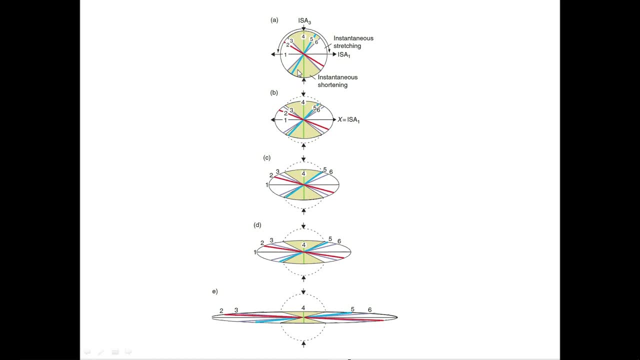 This creamy one is showing the regime of shortening, while this white one is showing the regime of extension. So, whatever the material line which is the shortening, Whatever the material line which is falling in this creamy region will deform to give fold, while the material line in this white region will deform after deformation will. 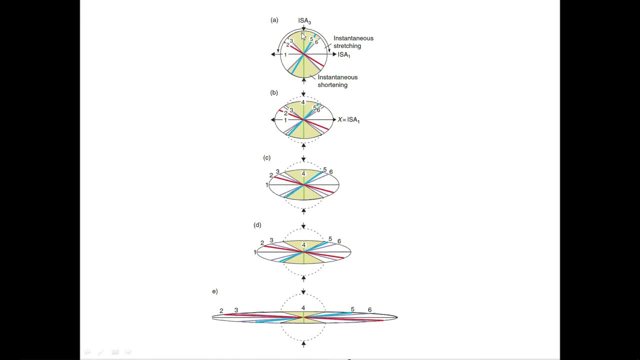 yield budinage, Although the maximum intensity of the fold will be in the material line, which are parallel to the instantaneous stretching axis, instantaneous shortening axis, ISA three, that is, parallel to the green one for line four. Okay, While the maximum extension, the maximum extension which is taking place parallel to the line, 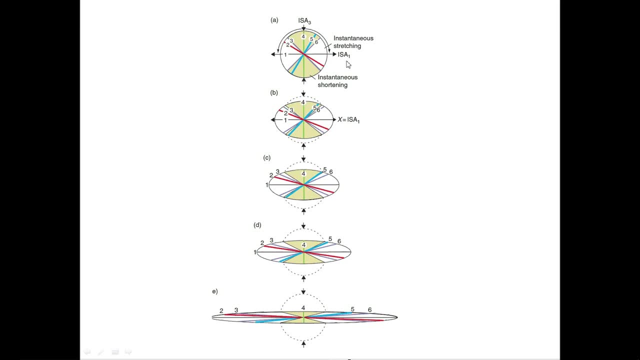 one ISA, one instantaneous stretching axis, one. Okay, So they will form the the most intensity of the budinage. the most intense budinage will be formed will be parallel to the line one. So here we can see as the strain is being accumulated. 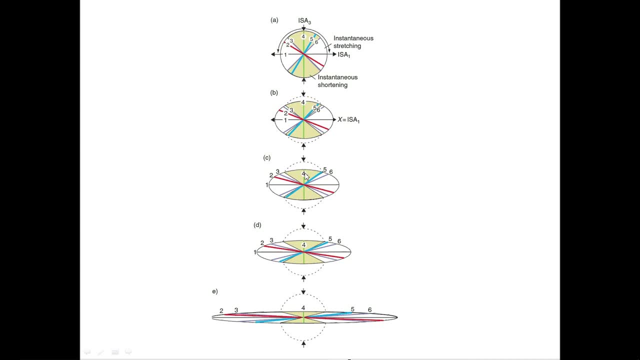 There will be no rotation of these Line four and one. Okay, As you can see, there is no rotation of the line four and one. They will remain at their same place. Okay, Moreover, there is no rotation of the ellipse, also, You can see. 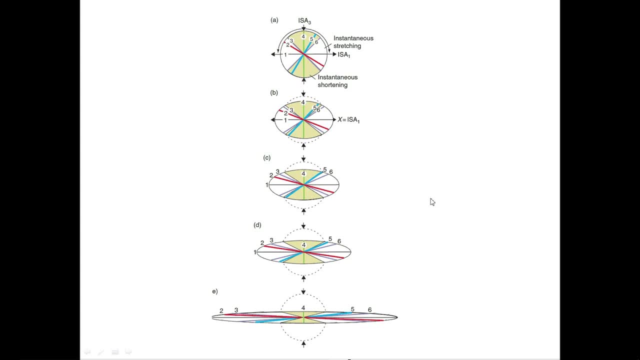 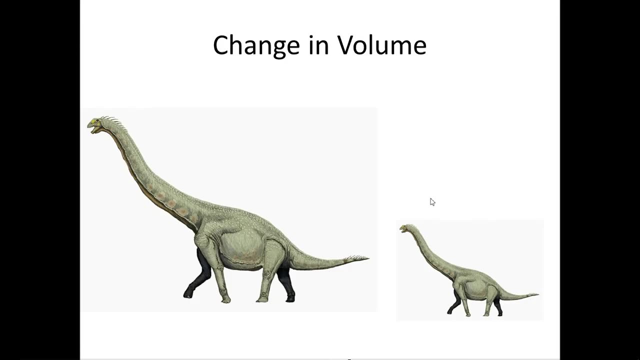 So this is an example of coaxial deformation, And at last, let us come to the last kind of deformation that we may encounter is change in the volume. Here we have a sauropod dinosaur. These both look identical, but one is very large in shape and other is very small in 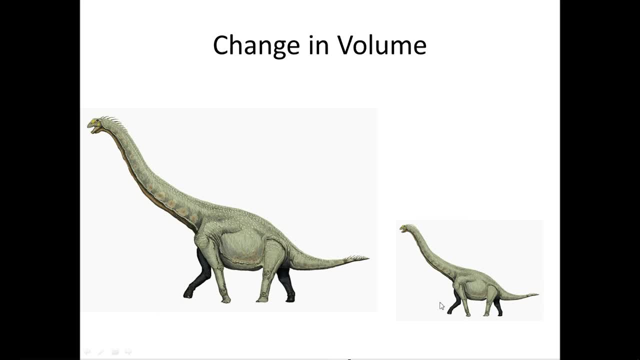 say very small in size, Okay. What is the basic difference between these two, these two animals? There is only one difference. that is their size. Okay, Their size and volume. If I made this this big dinosaur and shrink it to this of this dimension. 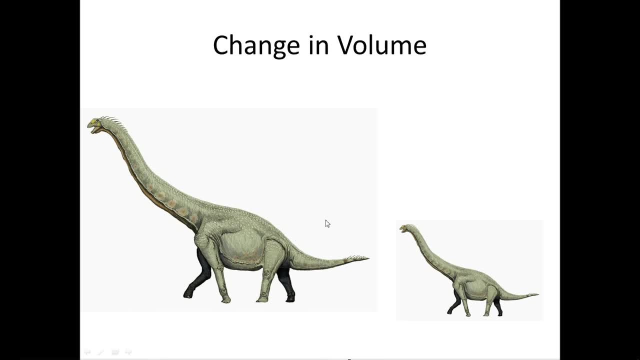 Okay, So there will be no distortion with the shape, because it there is no distortion of the face of the dinosaur, Neither it has any deformation: its neck, body, tail. No deformation in this region. Okay, So there is no deformation in the shape. 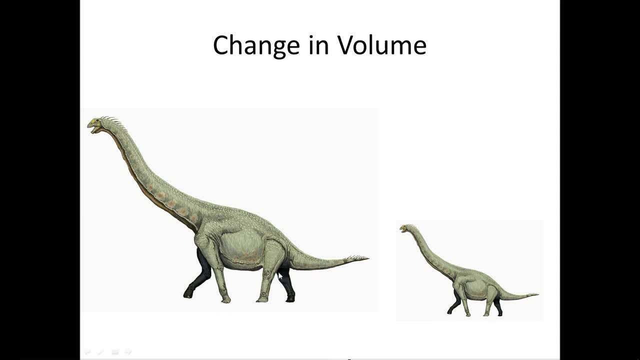 So we cannot call it the distortion of shape. Moreover, it is no rotation. No translation is taking place, So the only deformation is change in the volume. So just volume is being changed, Okay, Because of the change in the dimension. Okay. 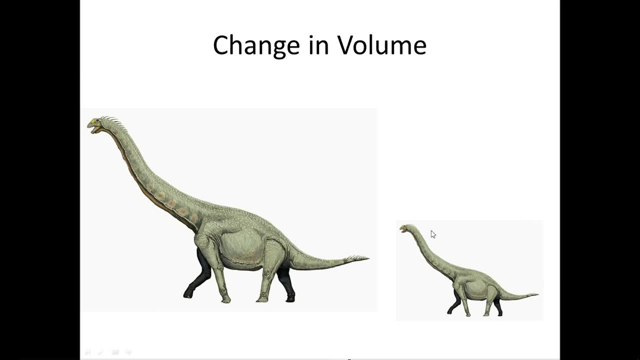 So its length, width, height is being changed and change in this dimension equally, in the equally, in equal proportion. okay, so when change in the dimension in the equal proportion is taking place, so the change in the volume take place. and the best example is: and the hydrostatic pressure. so hydrostatic pressure is a pressure. 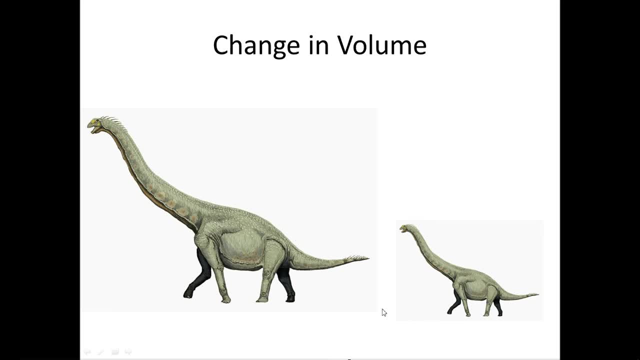 where, when you immerse body in deep under the water, what happens? that body got reduced in volume. there will be no reduction in the shape, no reduction. there will be no translation or rotation, rather there will be the body got shrink. so it's only only change in the dimension or change in the volume. will